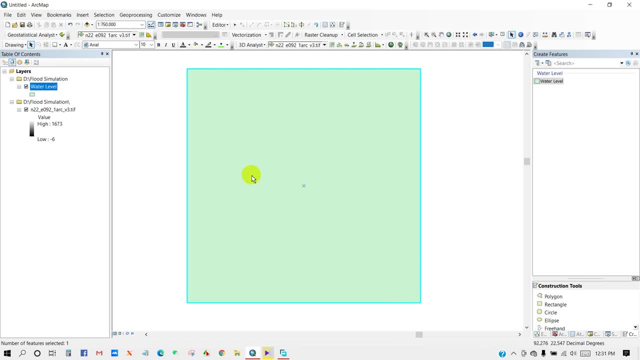 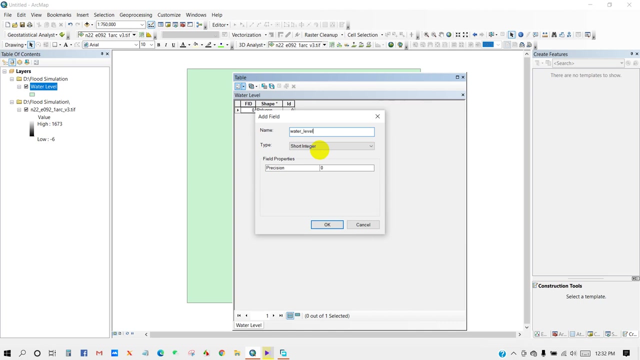 The shapefile is for water level, and then go to attribute table. I'm going to add a field, So first I have to stop editing And then And then go to here and then add filed And I'm going to name it as water level. 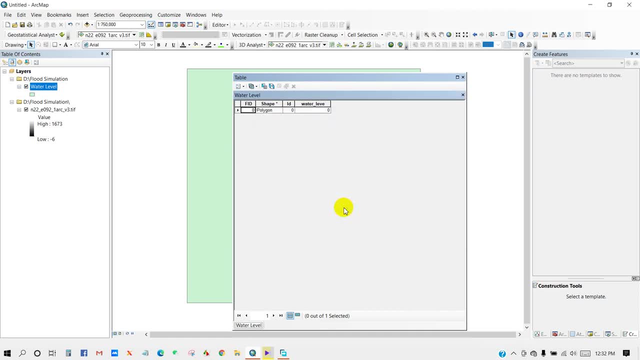 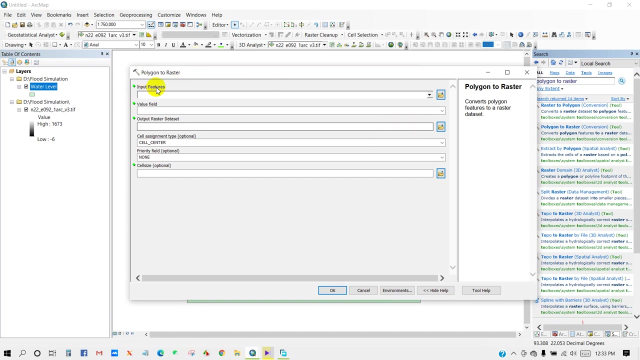 Click okay And again start editing. and water level. So the lowest order level, I mean I've made lower lowest elevation minus 6.. So I have just written here minus 6 about min C level and then go to search box and write polygon to raster. Actually I am going to convert this shapefile as raster, then polygon to raster and add water level shapefile as input features here and value field. 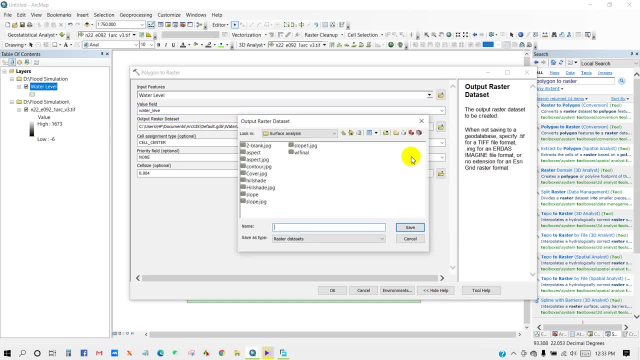 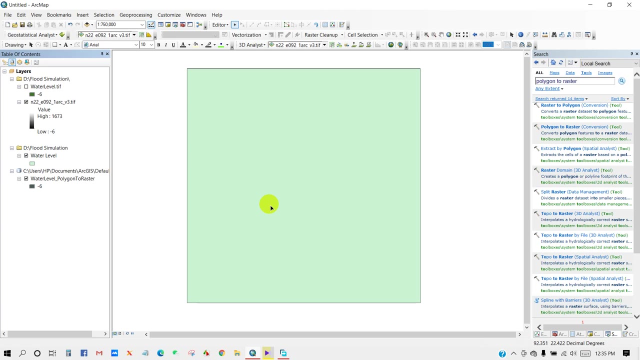 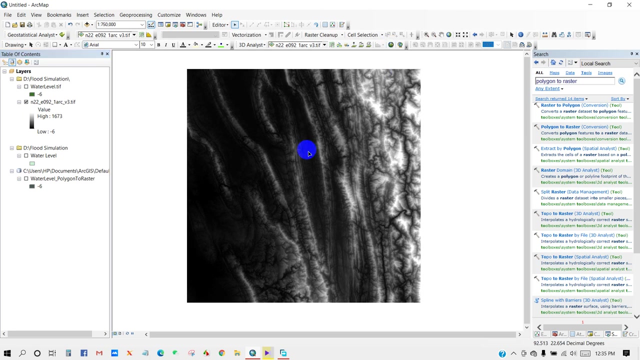 I am going to select water level as value field and output raster. Select a path where you want to save your file and then rename it. So I am going to name it as water level and then click save. So our water level raster has been generated and then go to arc scene. 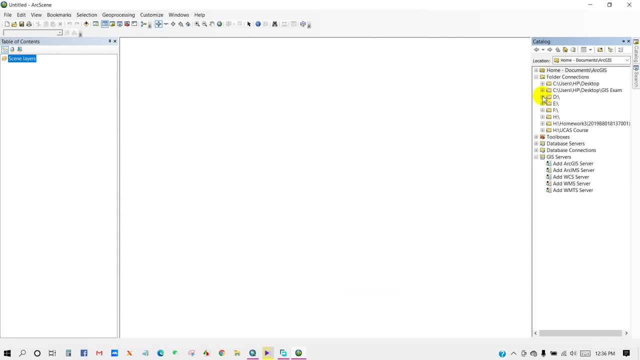 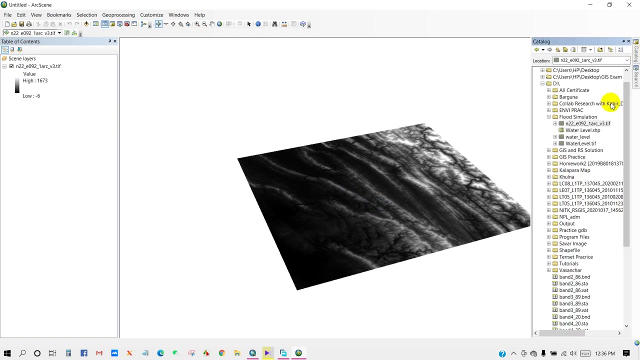 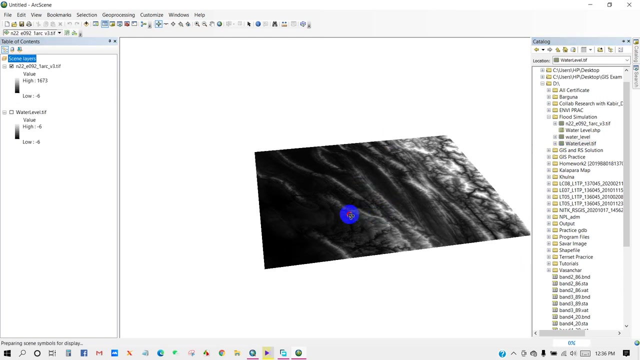 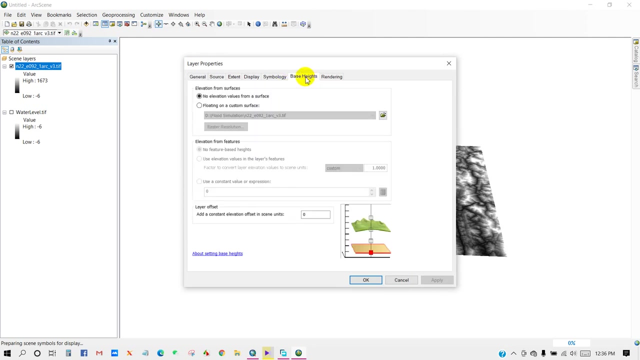 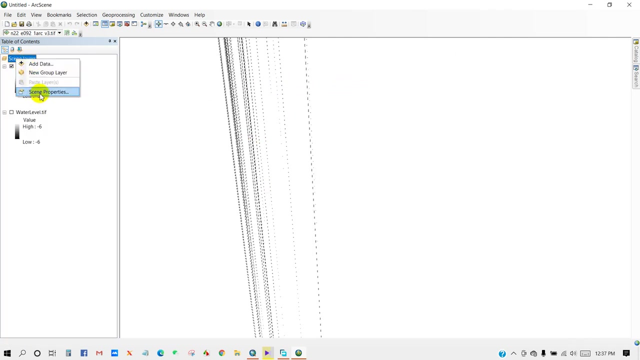 Navigate your folder where you have your file. So I am going to drag this file and drop here and the water level. click on the dim file, then go to properties and then base heights and check floating on a custom surface and then click OK. so after that it looks like that and then go to scene. 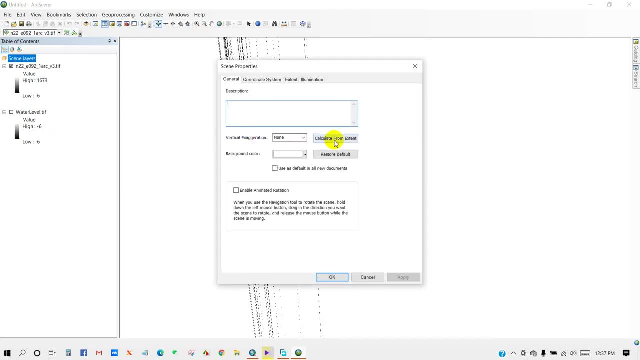 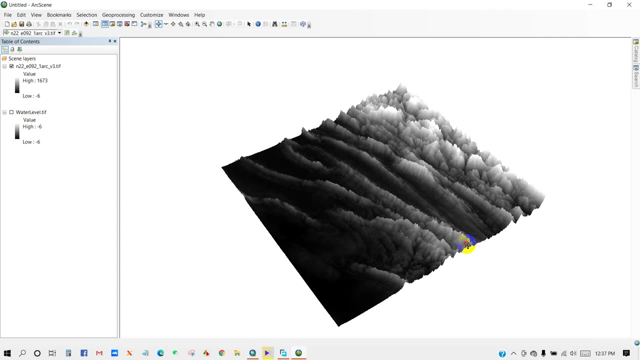 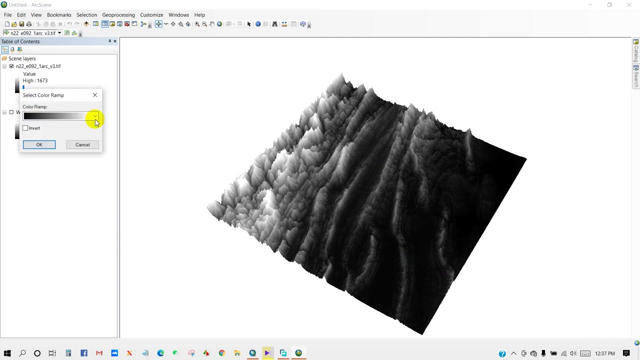 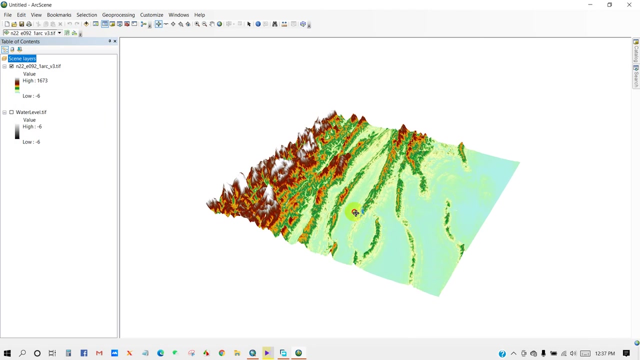 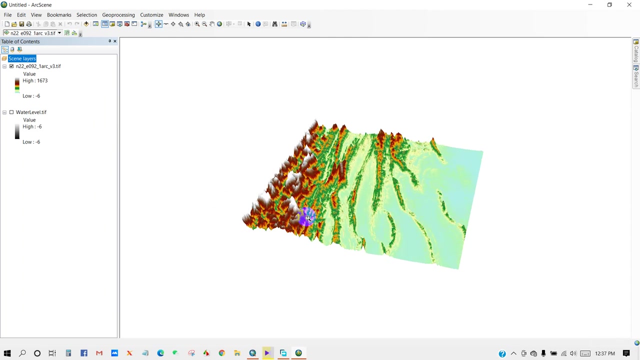 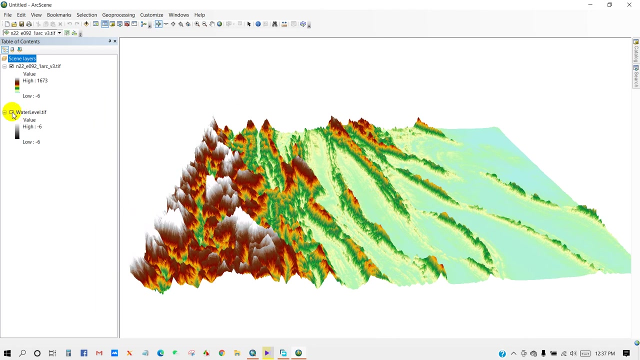 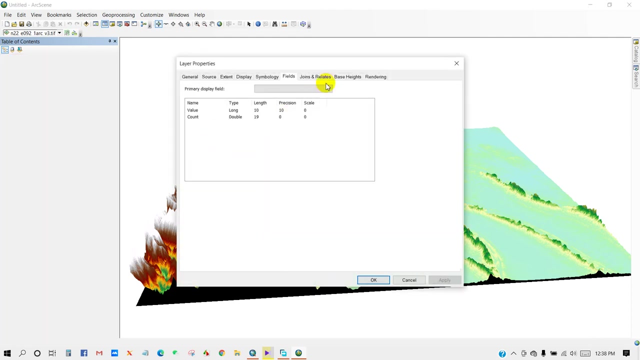 properties and then vertical excretion, calculate from extent and then apply. and okay, so now I'm going to change the color ramp, then click OK. the next step I'm going to do is so: here is my water level, you can see here. then go to properties and then symbology, and I'm going to give the unique value, change the color. 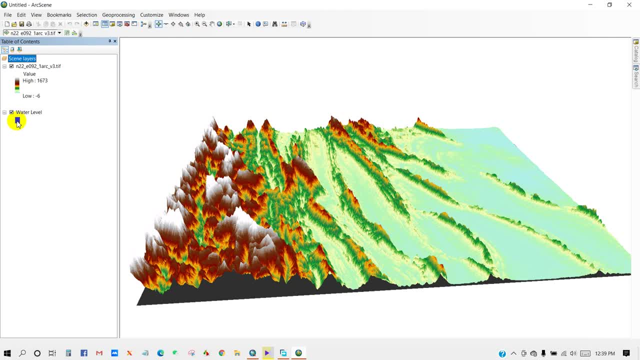 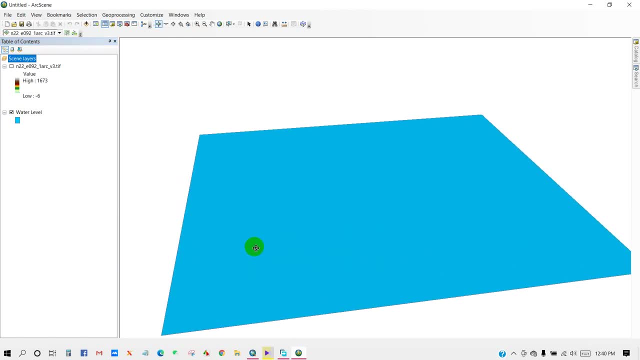 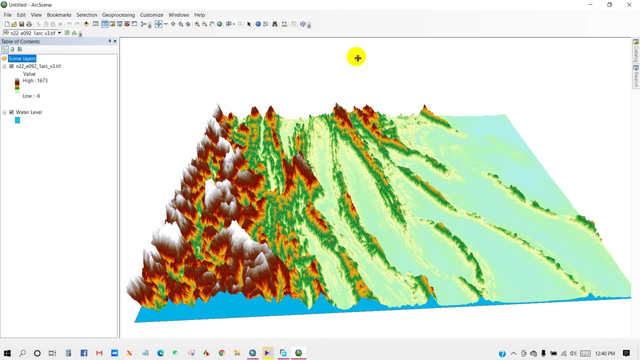 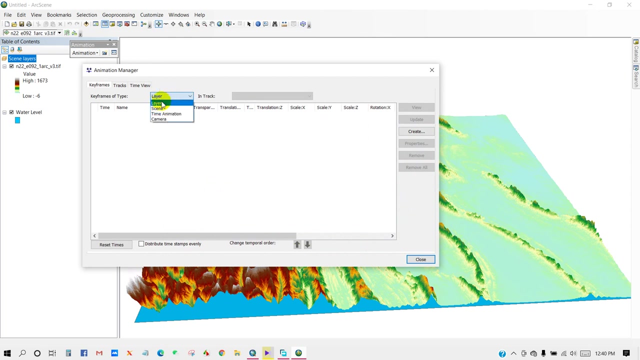 then okay, so click here and then animation, then go to animation manager and here select layer and then go to create and create animation keyframe- here source, object as order level, and then click new and here keyframe layer keyframe, so you can create a keyframe as. 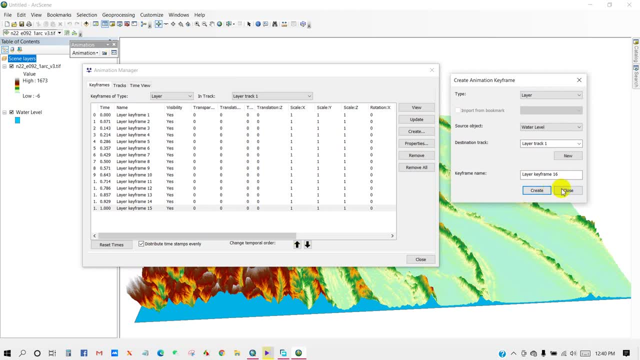 many as you would like to have, and here you have to give some values like specify how fast water level layer is going to rise up. so I'm going to write here: 10, 20, 30, 40, 45, 50, 60, 65, 70.